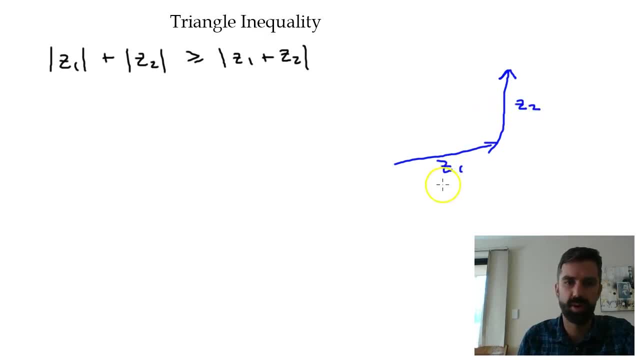 We add z2, the mod of z1 is the length of this line and the mod of z2 is the length of this line. So to get from here to here, one way of going is to take this entire vector and then this entire vector or the shortcut is actually my pen isn't great here. the shortcut is the vector that represents z1 plus z2.. 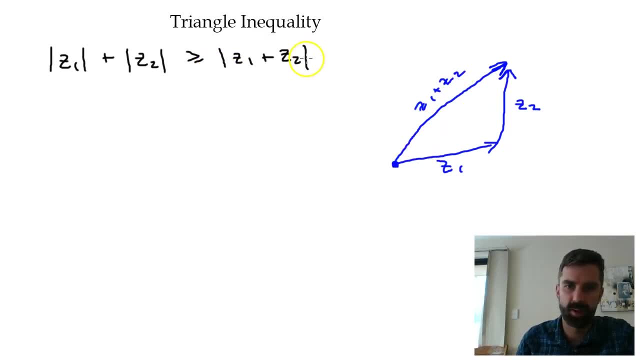 So what the triangle inequality is actually saying is that it's always longer, in terms of distance, to get from here to here by taking z1 and then z2 than it is by just taking the direct route. Now note that it's greater than or equal to. The case where it's equal to is when z1 and z2 actually lie on the same line, so their arguments would be the same. 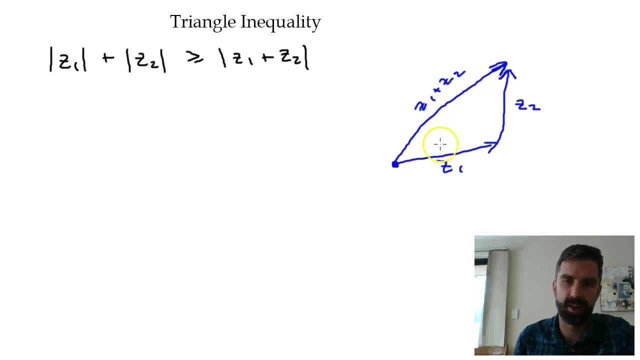 And so then you're just sort of travelling in a straight line regardless. So that's what the triangle inequality says. So we've shown that's true. Now, what we didn't really get a chance to look at is what I would call the generalised triangle inequality. 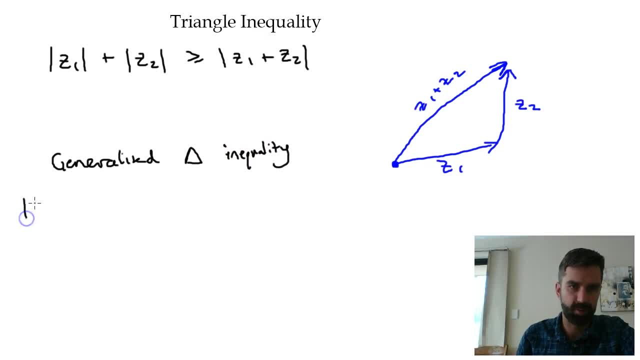 And that basically says that we can take this out to any number of complex numbers. So z1 plus z2.. z2 plus a whole bunch of complex numbers up to zn. If we add up all their moduluses, moduli, that's going to be greater than or equal to the modulus of all of them added together. 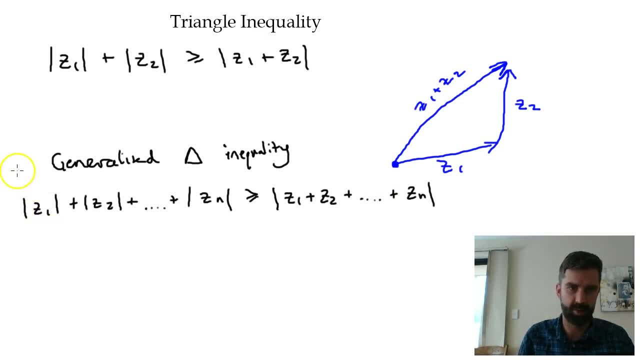 So we're going to prove this by induction. So if that's our pn, let's prove p1 first of all. Well, if it's p1, we've just got z1. And that's going to be greater than or equal to the mod of z1 on the other side, because they're equal. 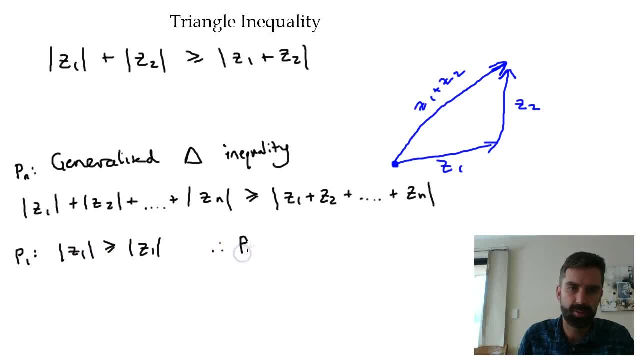 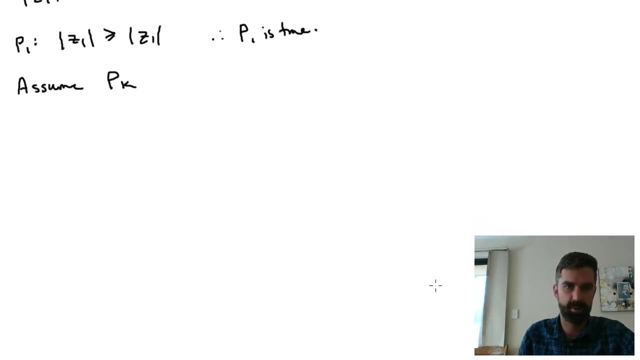 So it meets that condition of equality. So therefore, p1 is true. That's lovely. Now what we're going to do is assume pk, And I'll just move down to here. So pk, pk says that z1 plus z2, plus a whole bunch plus zk, are going to be greater than or equal to the mod of all of them added together. 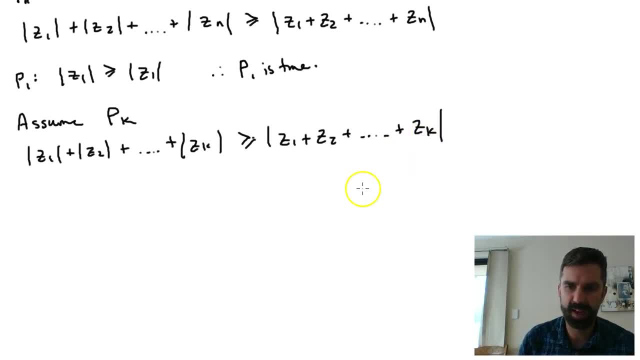 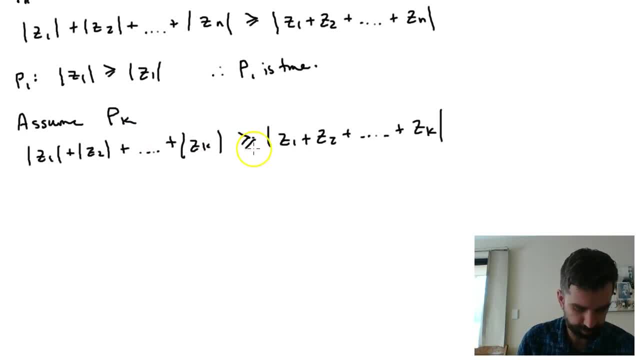 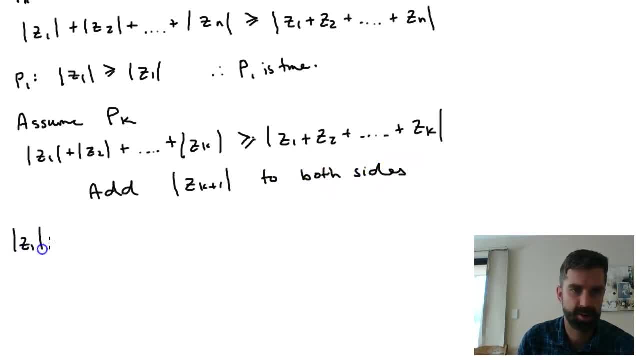 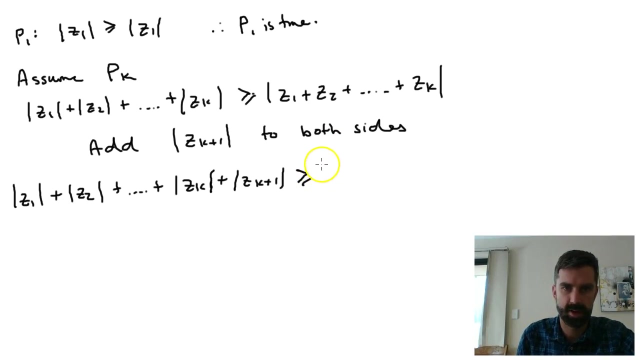 So that means that the left-hand side becomes the same thing up to zk plus zk plus 1, and that's going to be greater than or equal to the mod of z1 plus z2 plus zk and then plus the mod of zk plus 1.. 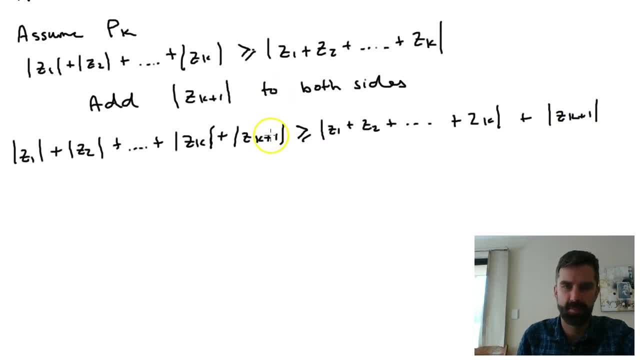 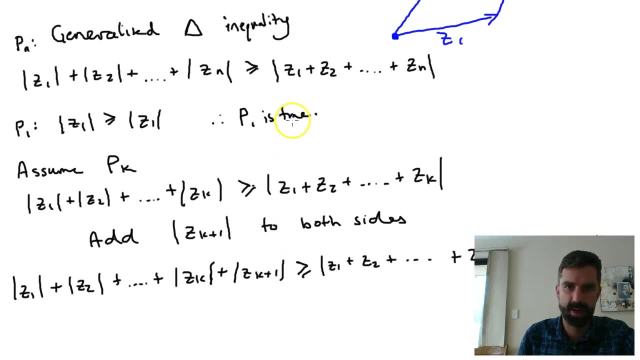 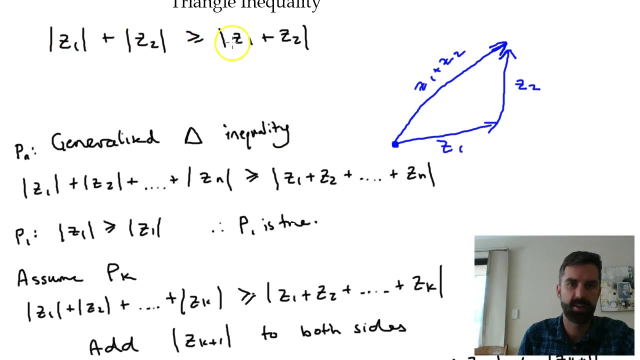 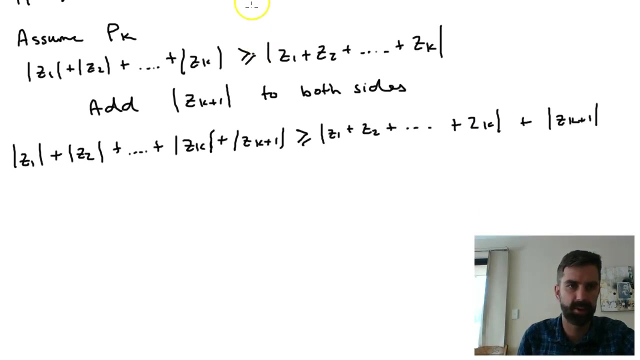 Now we've got to think back to what we already know about the triangle inequality. Our original triangle inequality, just for a regular triangle, says that the modulus of two complex numbers added together is going to be greater than the modulus of those two complex numbers added. So if we go back to where we're up to here and look at the left hand side, 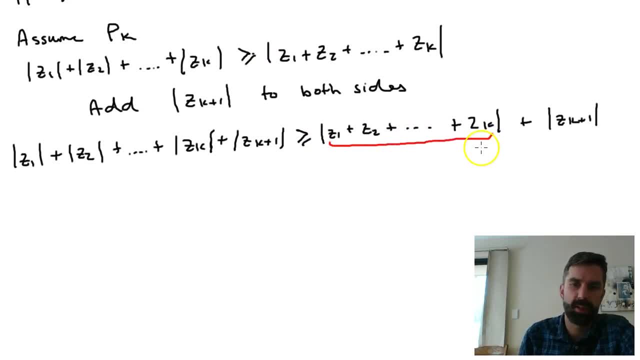 whatever this is, this is some complex number. It's going to be some sort of complex number. Here's another complex number and we're actually adding the modulus of those two complex numbers. So we know that if we add the modulus of these two complex numbers together, that's going to be greater. 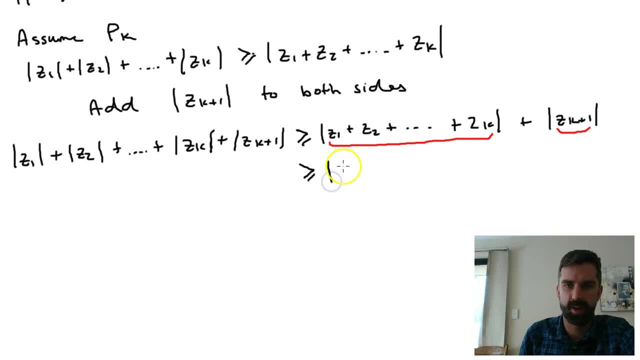 than or equal to the modulus of this number plus this number. So that means we can actually say that this is greater than or equal to that complex number plus that complex number based on the triangle inequality that we've already proved. And if this statement is greater than or equal to this, 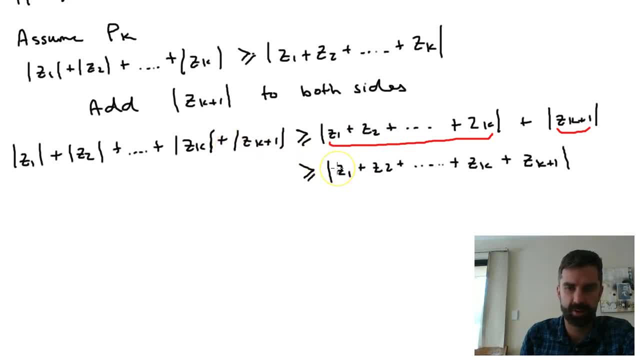 statement. well then, this is also greater than or equal to this. So what we've actually shown is that pk plus zk is greater than or equal to this. So this is greater than or equal to this plus one is true, if PK is true. So relatively simple induction proof What it relies on. 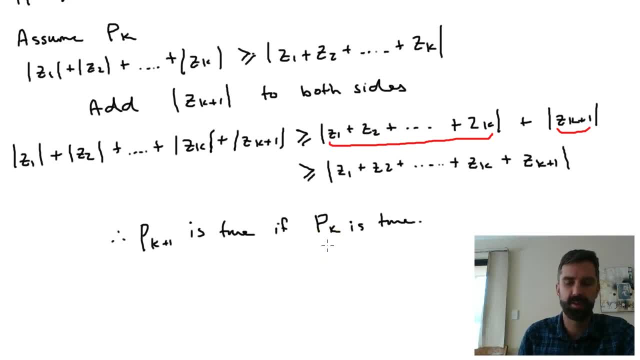 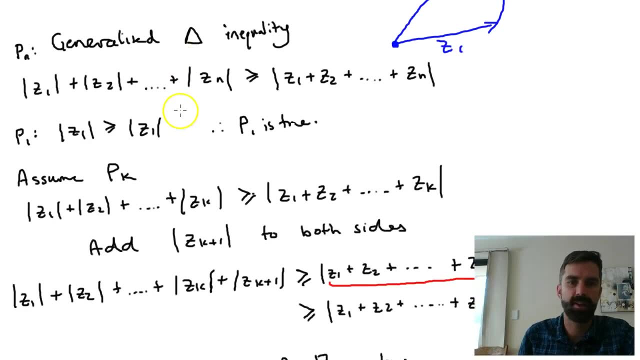 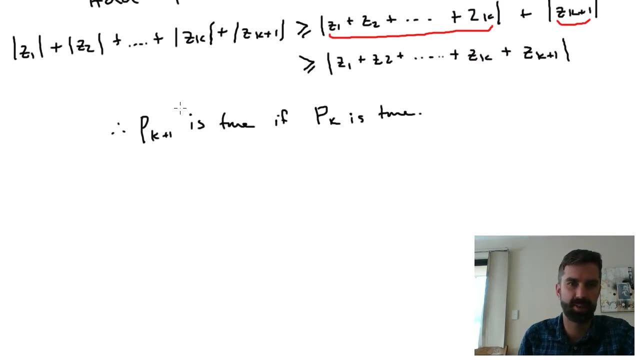 and this is true for most of your induction proofs of complex numbers- is taking the case that we've already proven for two complex numbers and then applying that to the case where we've got n complex numbers, And that's often the way that you get these complex number proofs to work out. 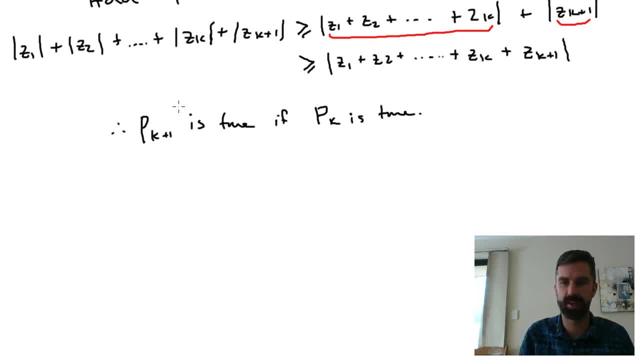 because you can prove it for two complex numbers using either vector geometry or by letting them equal a plus bi, any sort of technique like that- and then you can apply that to your generalized inequality. Just one more thing, just thinking about what this generalized inequality means. 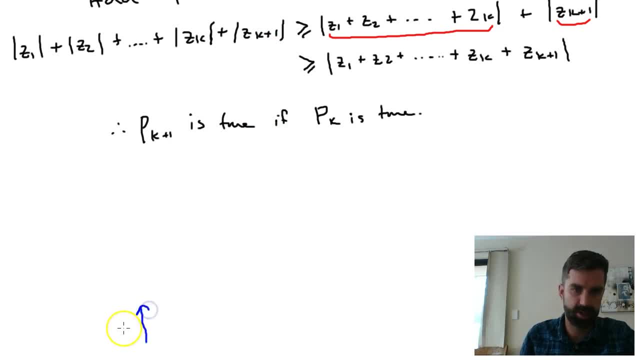 well, what it actually means is if you've got, say, z1,, and then you add on z2,, and then you add on z3,, and then you add on z4, and so on, let's say n is equal to 6, and we end up doing this.